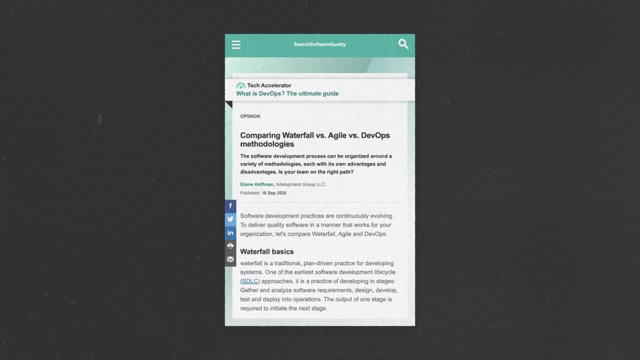 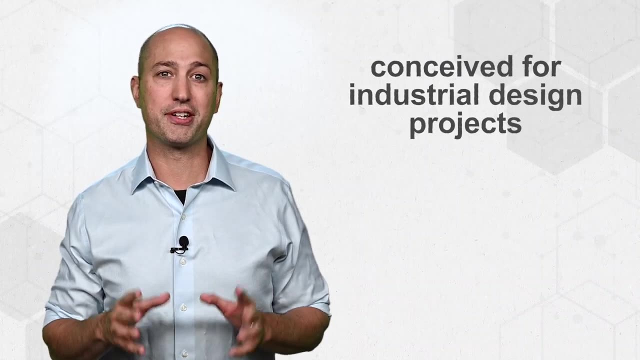 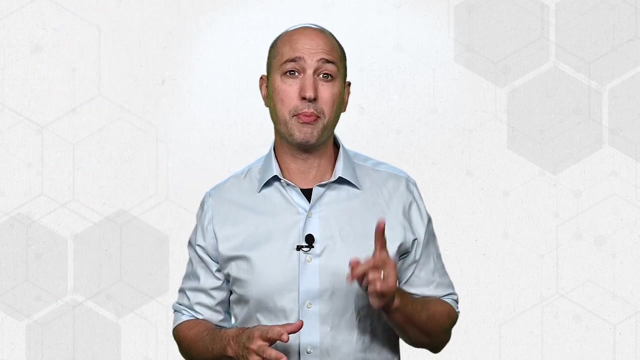 up against other methodologies like Agile and DevOps, and hit the button in the corner to subscribe for more videos on all things business tech. The waterfall method was conceived for industrial design projects, but software engineers often use it today. The method consists of seven phases, each of which must wait for the previous one to finish before starting. The phases are: 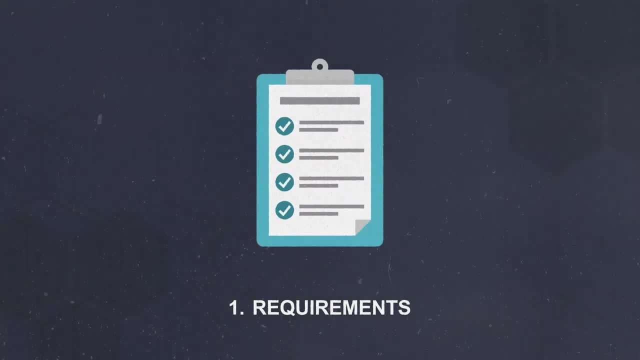 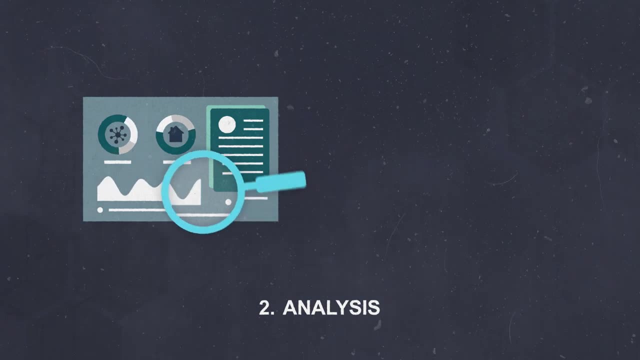 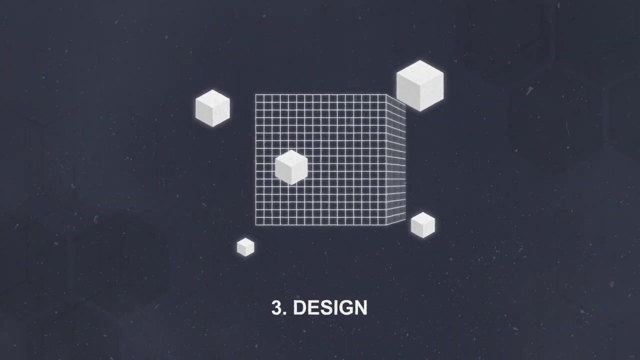 requirements. Customer requirements are gathered. This generally, is the only time customers can provide input. Analysis System specs are checked to make sure they'll work in production, and financial and technical resources are required. Design Technical requirements are outlined, including the programming language. 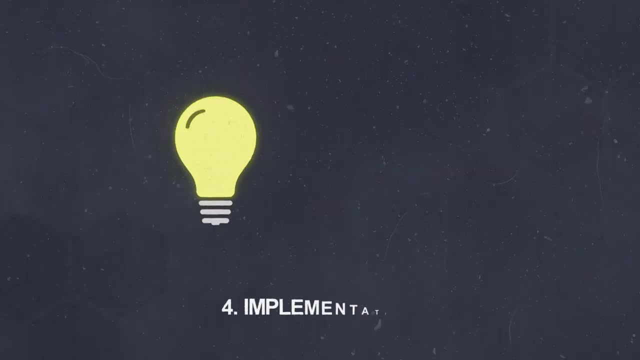 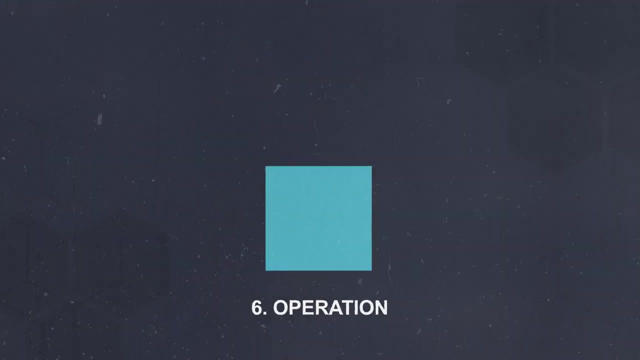 architecture and hardware to be used. Implementation: The design is implemented and production begins With programming. the source code is developed in this stage. Testing: Quality assurance and other tests are applied and debugging takes place if needed. Operation: The product is deployed to the customer. 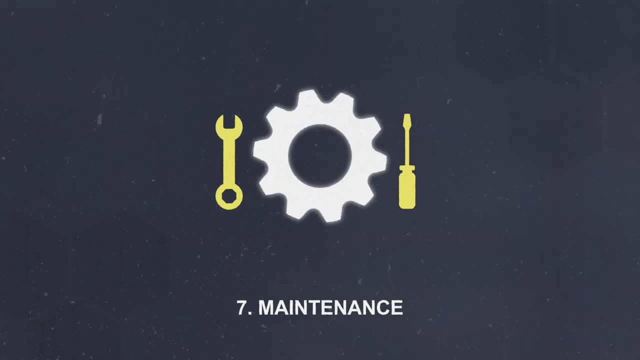 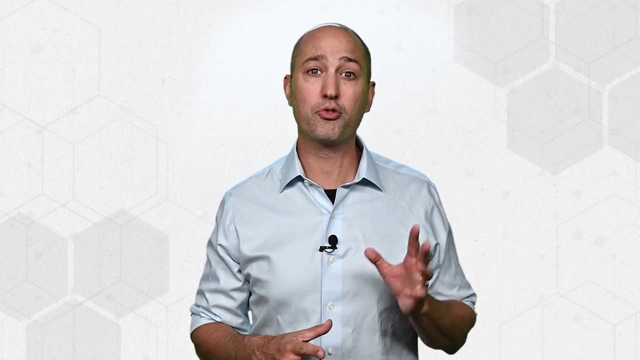 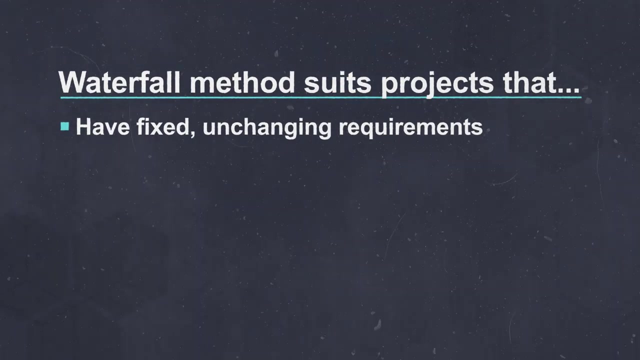 Maintenance, The product is maintained and supported. In software development. this is where the software patches are applied. The waterfall method lets development teams move efficiently through the phases of a project without much input or interruption. This makes it suitable for projects that have fixed, unchanging requirements require specific documentation. 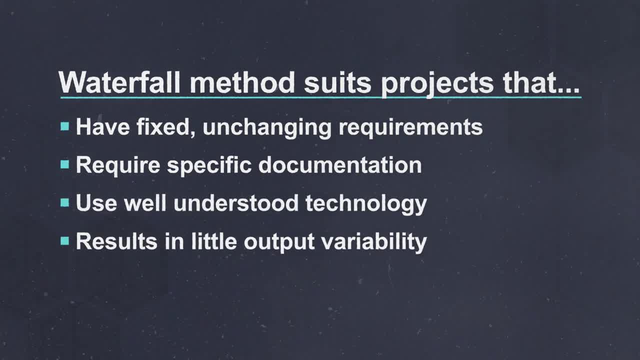 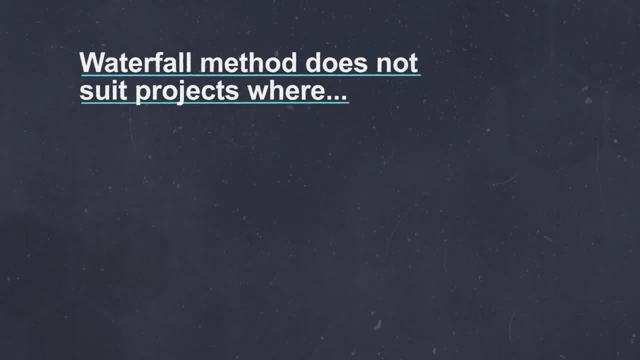 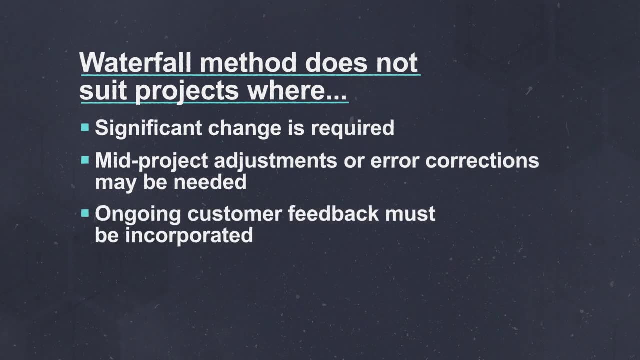 use well-understood technology, results in little output variability and must work on the first try. The waterfall method isn't ideal for some projects, such as ones where significant change is required. Mid-project adjustments or error corrections may be needed. Ongoing customer feedback must be incorporated. Two processes are performed simultaneously. 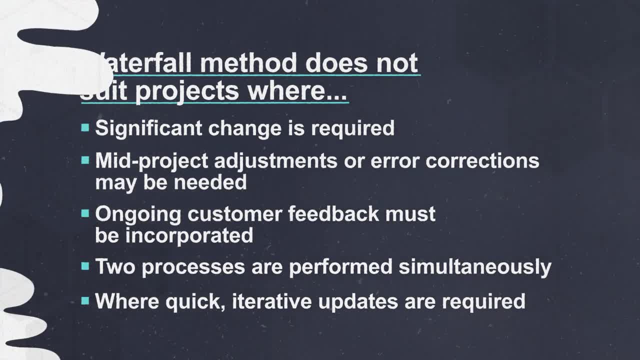 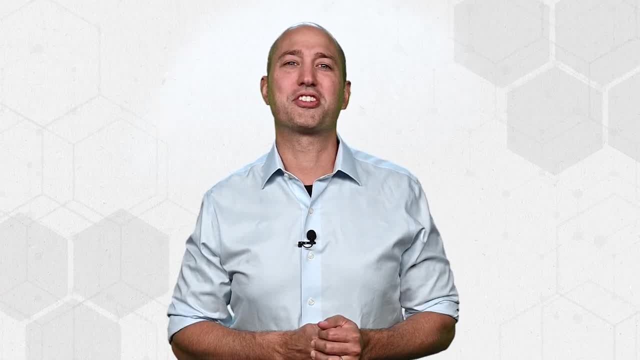 or where quick iterative updates are required. Development teams may choose other methodologies, like Agile or DevOps, because of the increased flexibility they allow. Which methodology does your team use? What is waterfall method best for? Let us know in the comments below, and be sure to hit the like button and subscribe too. Thanks for watching.